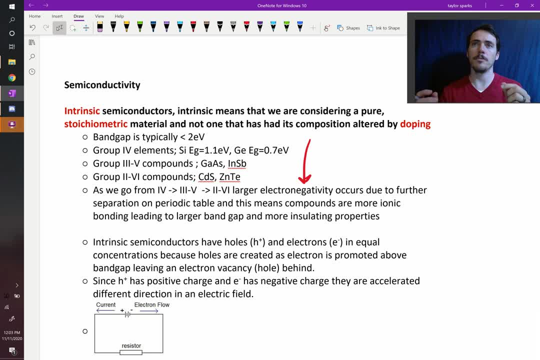 three, five, two, six. what you're seeing is you're putting a bigger difference in electronegativity. right At group four, they have the same electronegativity. Group three, five, there's a little difference. Group two, six, it's a big difference As you increase the 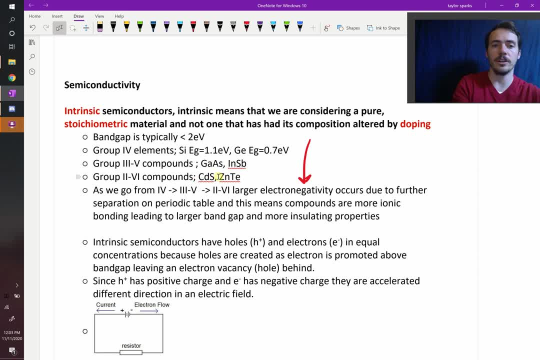 difference in electronegativity, you make the bond more ionic. right, It becomes more ionic and therefore it's a stronger bond. So you're putting a bigger difference in electronegativity and so the band gap increases. So your intrinsic semiconductors are going to be the most. 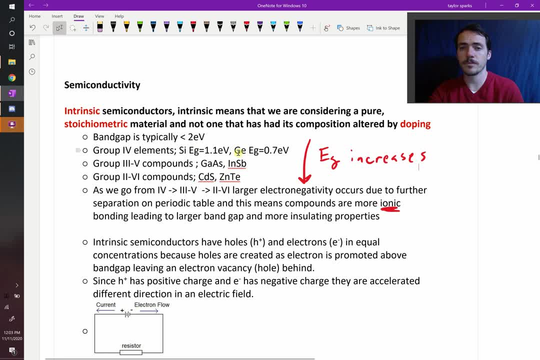 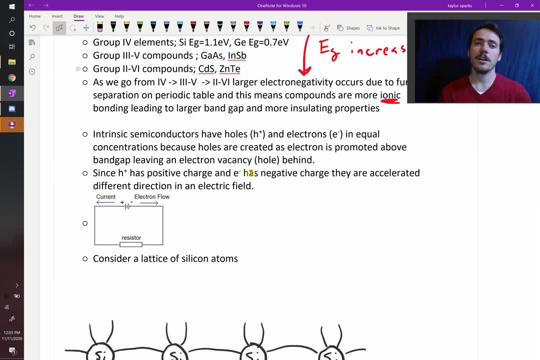 conductive for silicon and germanium because the gap is small and the least conductive as you move down this series. okay, Another thing to note about intrinsic semiconductors is that the concentration of your holes in the valence band and your electrons in your conduction band are 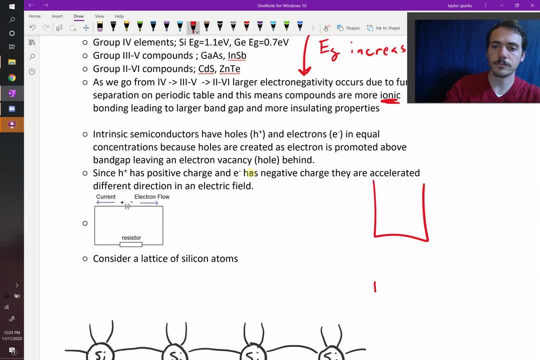 equal because if we draw our picture here, the Fermi level is right, smack dab in the middle for intrinsic semiconductors. So for every electron that was down here- right, this was filled with electrons- for each one that you create a hole like, let's say, four of those get created, you put. 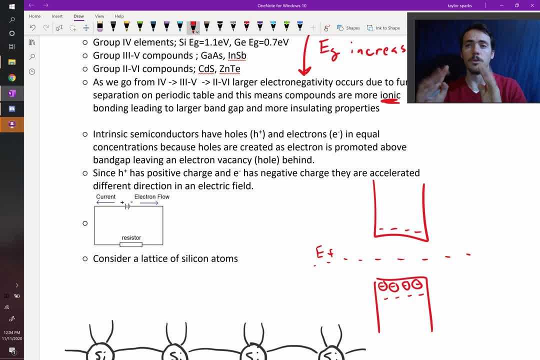 four up here. So now you have four electrons and you have four holes. okay, So they're in equal concentration for intrinsic semiconductors. And what's cool is that both of these are available for conduction, right, If you think of, like our schematic for electrical conductivity in a circuit. 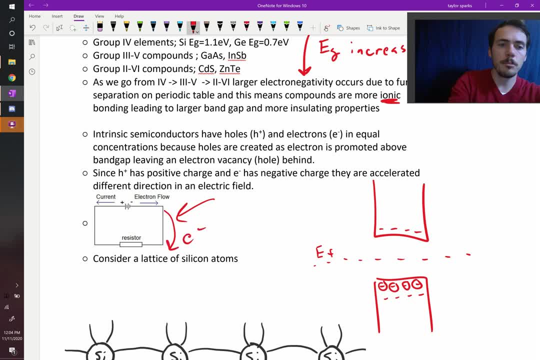 you have electrons traveling this way- right, But that means if you're current is going that way, what you're really having is your holes travel that way. So these will travel opposite directions, but they create current in the exact same way, Like it's the same. 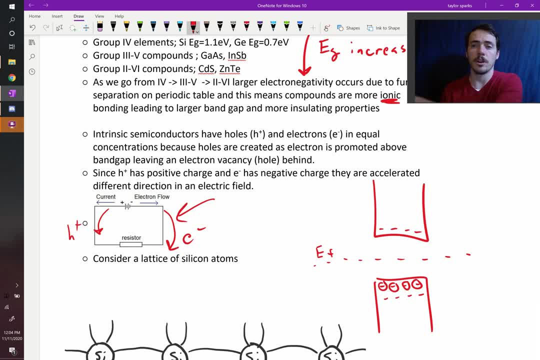 current. the current is the same direction, but your electrons, which are negatively charged, go one way and your holes, which are positively charged, go the other way. right, But they both contribute to the electrical conductivity. I think it's useful to think about intrinsic 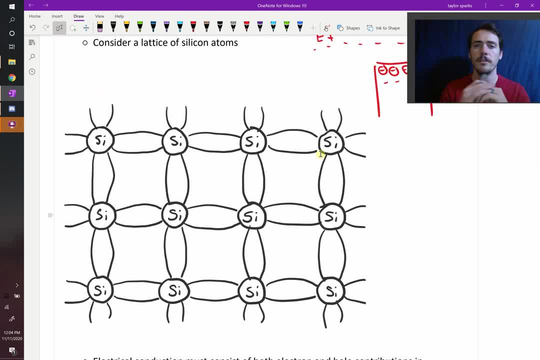 semiconductors by picturing this lattice of silicon. Let's imagine we have pure silicon, right? We know that silicon is bonded to four other silicons and it is not flat sheet. I'm showing it as a two dimensional plane here, but we know that this is actually a three. 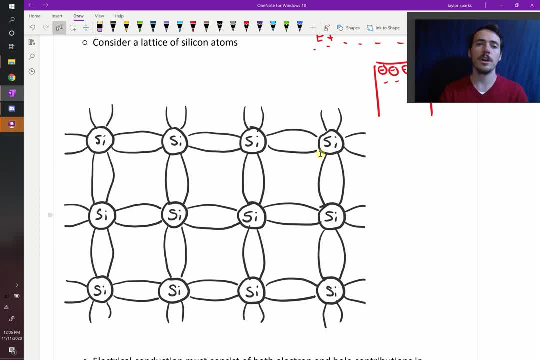 dimensional diamond cubic lattice. But consider this for a minute: What do we know about each silicon? We know that each silicon has four electrons, right? So if we start drawing these, this has one, two, three, four. there we go. Every single silicon had four electrons, And so 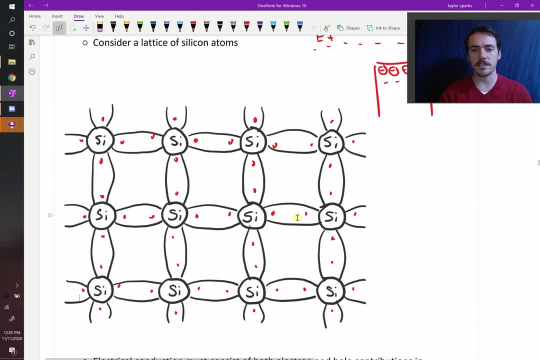 by all sharing, they end up with one, two, three, four, five, six, seven, eight. They have a filled shell, and so they're happy, right? So what has to happen in order for us to get conduction right? 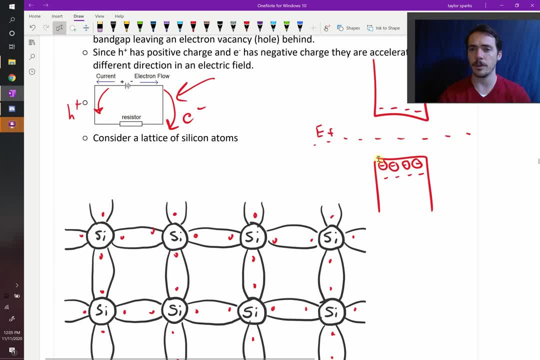 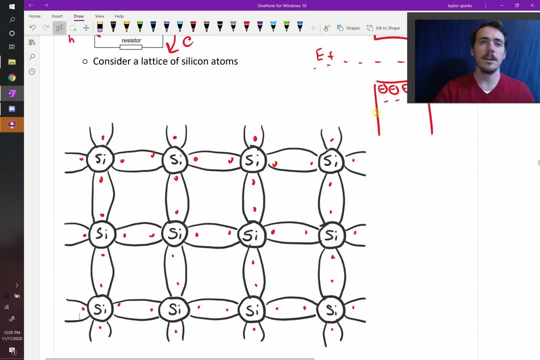 We had to promote one of these things from its filled shell, where it was happy right This filled valence band. We had to promote it across the band gap up to the conduction band. So what that looks like is we're literally taking one of these electrons right here and we're pulling it out. 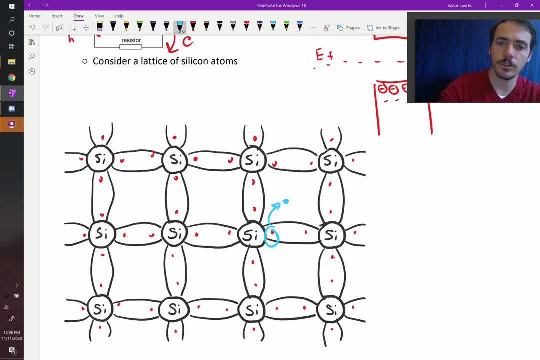 of that bond, right? So now this is a free electron which is negatively charged, and that created a hole, right? So now we have a hole which is positively charged and an electron which is free, And what that really meant is that we pulled it out of that bond and we pulled it out of that. 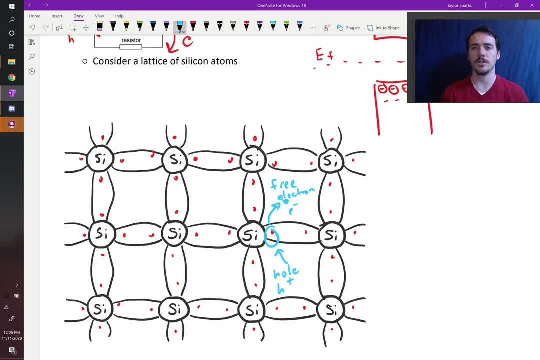 bond and we stuck it up in a higher energy level bond right, So it didn't have to physically move out of the lattice, It just went to a higher energy level. It's at the same position, just at a higher energy level. But what happens is when we apply an electric field across this. 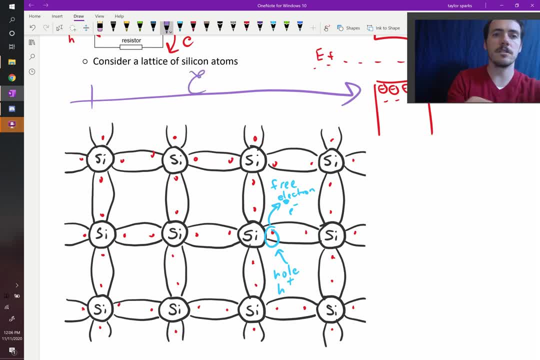 thing right. If we apply an electric field across this silicon, you know group of atoms, now these things which are charged, our hole and our electron are going to move in response to that field. The electron is going to travel this way and the hole is going to travel that way. 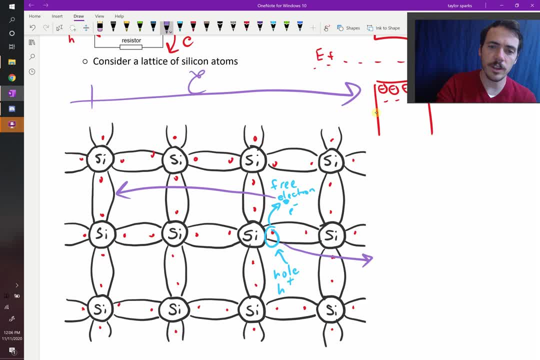 Now, how does the hole travel? It travels by the nearby electron coming and occupying that hole. and now the hole has moved to right here, and then maybe this one will occupy that hole, and now it's moved to there. So it moves by hopping in that lattice and the free electron is now in an empty. 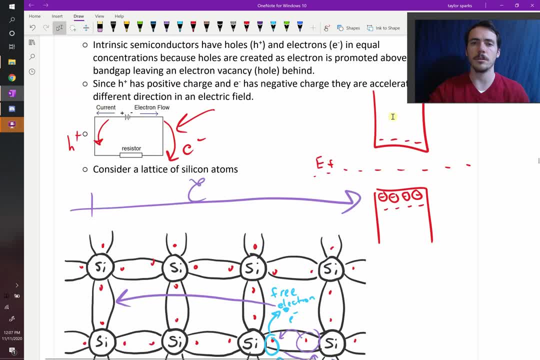 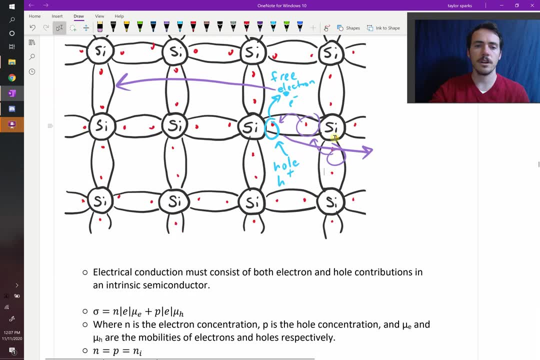 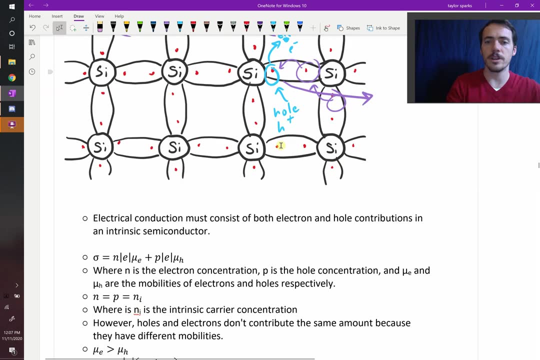 conduction band. So it just essentially moves without worrying about holes coming and an electron coming and filling the hole where it was okay. So that is intrinsic semiconductors Again, because every time we created an electron we also created a hole. we have the same concentrations, right, Electron and hole.